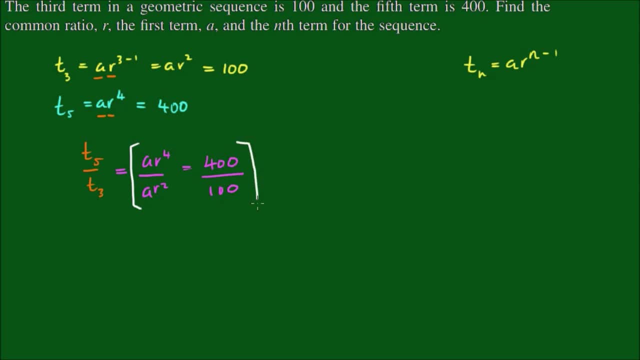 So let's just consider this part of this equation. I can cancel two zeros straight away on the right hand side And a cancels with an a, and that simplifies down to r: squared equals 4, which means that r- if we take the square root of 4, has two possible values. 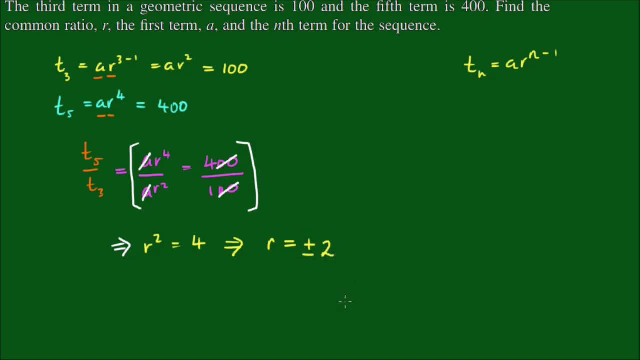 So positive or negative, 2.. Alright, so we've got two possible values for the common ratio, and that means there is two possible values, a positive or negative value, for each of the odd number terms, except for a positive or a negative number. the first term A, And now we can substitute this result back into. 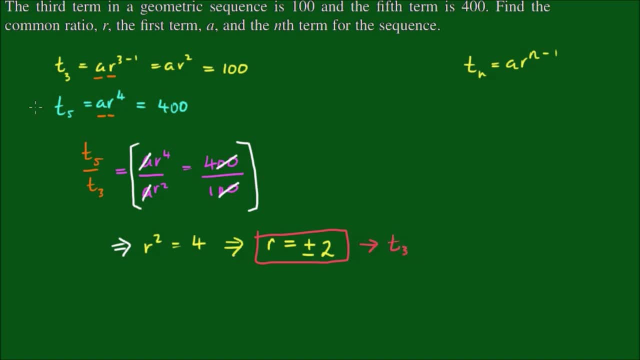 T3 to solve for A. So let's do that. We've got T3 equals A by R, which is positive or negative. 2, squared equals 100.. So that implies that A, if we do the calculation, positive or negative 2 squared. 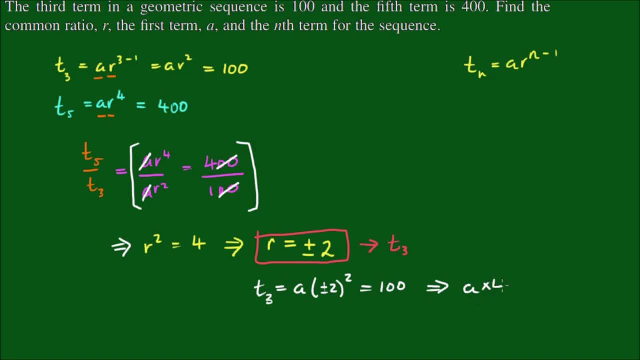 is always a positive, And that comes out to equal 4.. We've got A times: 4 equals 100. And therefore A is equal to 100. divided by 4 equals 25.. So this is our second piece of the puzzle. 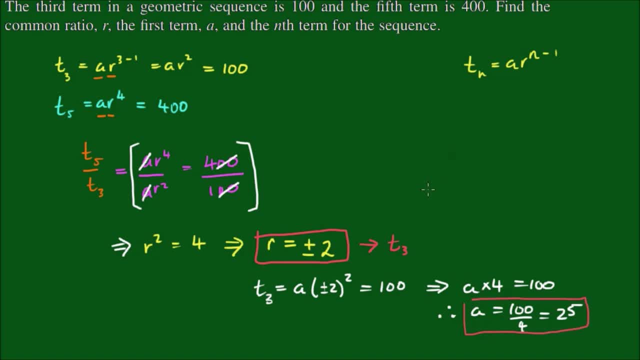 Finally, we're asked to find the nth term. So from here T, sub n, the nth term is given by A, which is 25, by R- I'm just going to leave it as positive or negative 2.. It doesn't look very elegant, but for convenience sake let's just leave it like that. 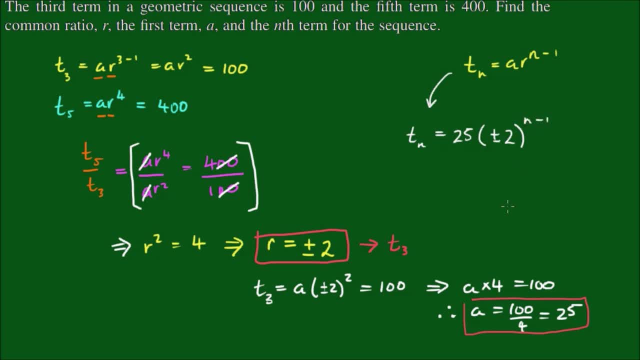 And then we have to the power of n minus 1.. Okay, so if we take the positive value for R, so positive R, the sequence will look like 25, the starting number, Multiply that by 2, the second term will be 50.. 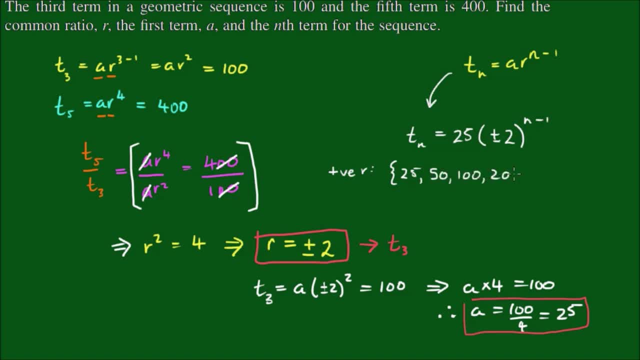 Third term is 100,, 200, and 400, and so forth. If we take the negative value for R, the series will look like 25.. Starts off with the same number. The second term will be negative 50. So I made a mistake earlier when I said: